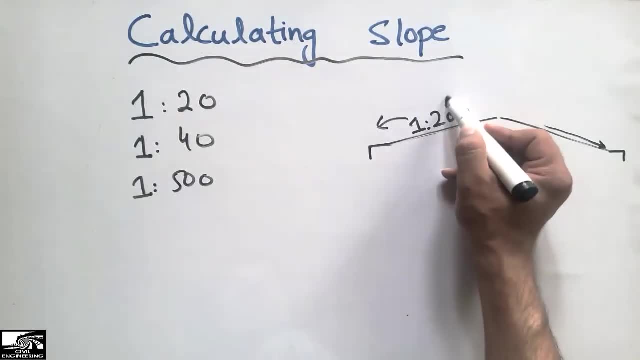 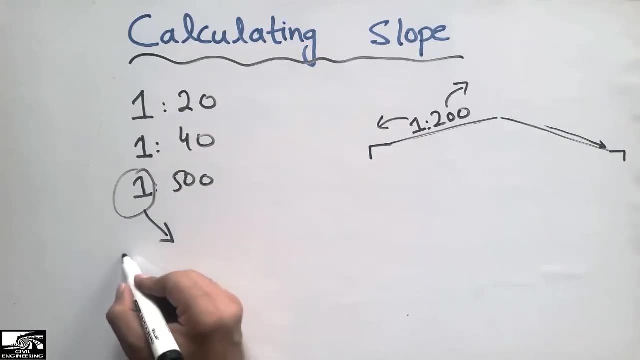 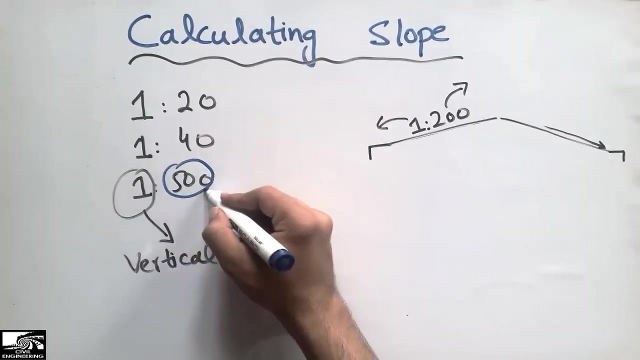 So what is the one value represent and what this 200 represent? The left side value. the left side value always represent the vertical portion of the line, the vertical portion right, While the right side value always shows the Horizontal portion of the line horizontal. 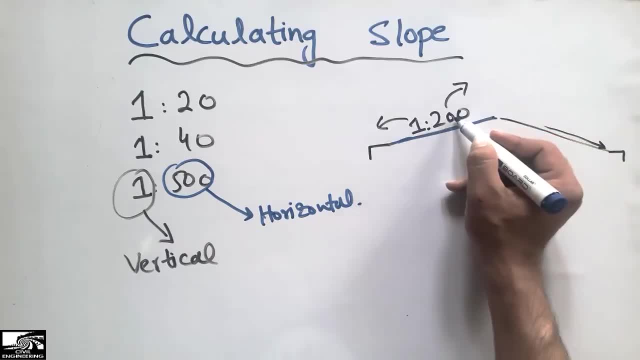 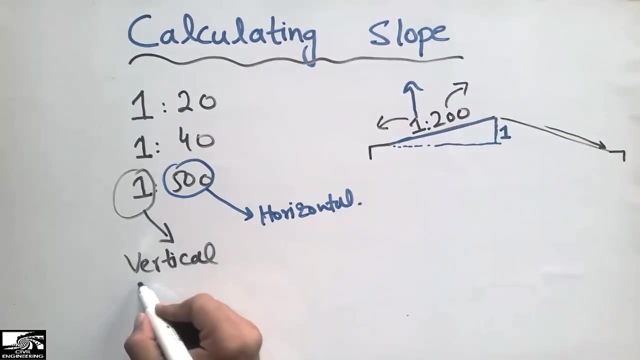 It means if this is the line having slope of 1, ratio, 200, it means that consider: this is the horizontal line and this is the vertical line of this line, vertical portion. So its vertical portion is 1, its vertical portion is 1, the left side 1 here, so I write 1, while the horizontal portion is 200, the right side is horizontal. 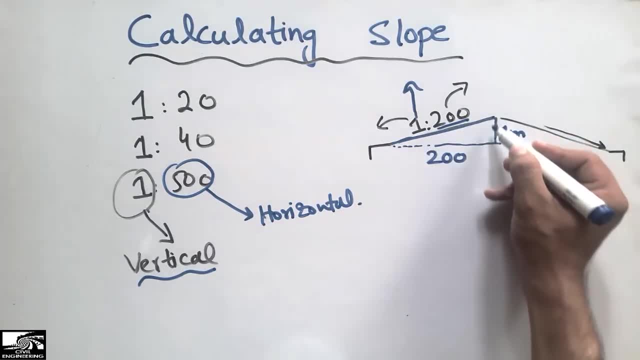 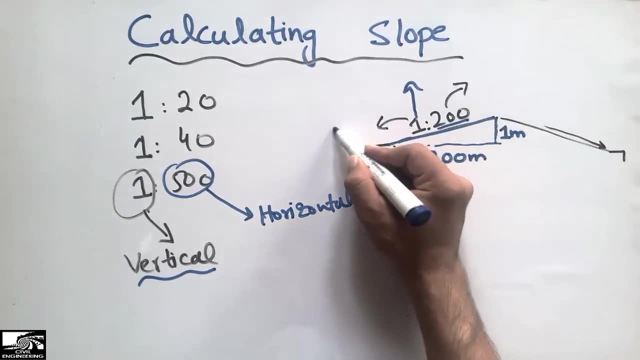 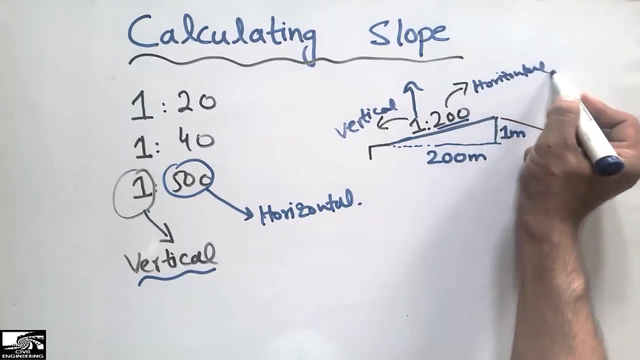 So it's 200,. it means if this is 1 meter high the line, so its horizontal distance will be 200 meter or length. This shows the vertical, while the right side value shows the horizontal. So this was all about the how we read the drawings. 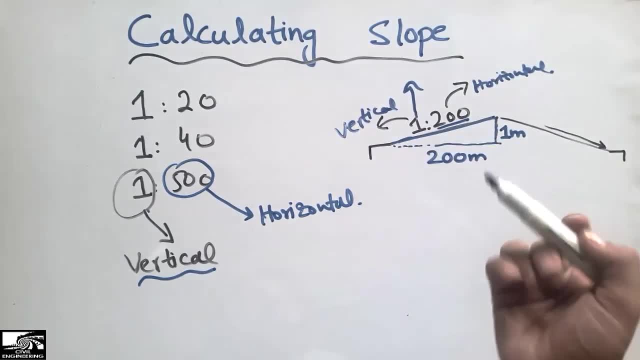 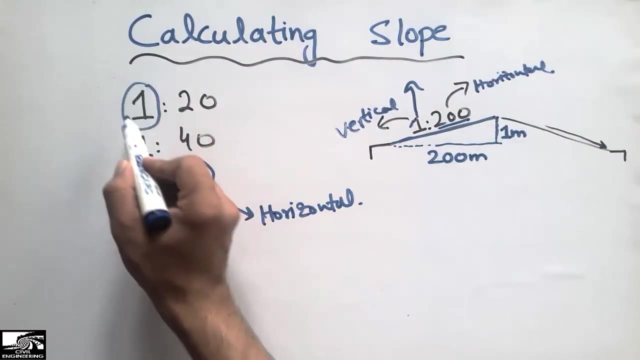 If the slope of any line or the intersection is given, so we can read these lines by knowing that this left side shows the horizontal length of the line And the right side value shows the vertical portion of the line. Similarly is the case with this value: The one is the vertical line. if I consider this is a line, 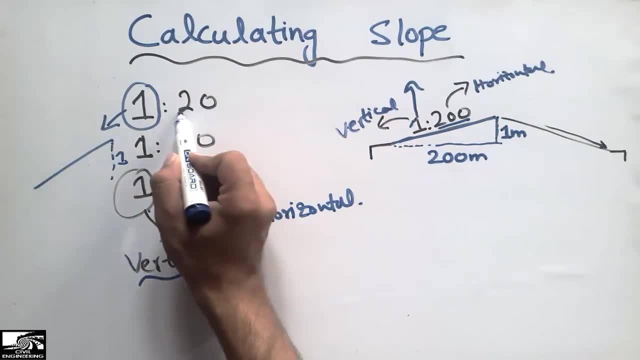 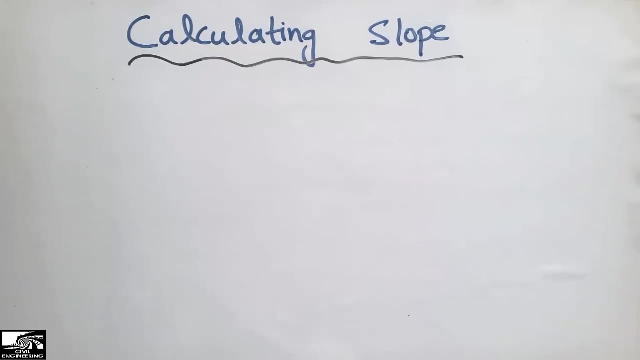 So one is the vertical line one here, while the 20 represent the horizontal length. It may be 20 foot, it may be 1 foot. So the one is a vertical foot, 1 foot, and the horizontal is 20 foot. Now I will show you how we find the slope of any given line. 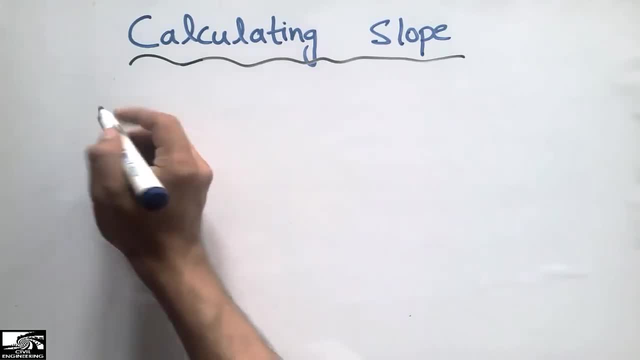 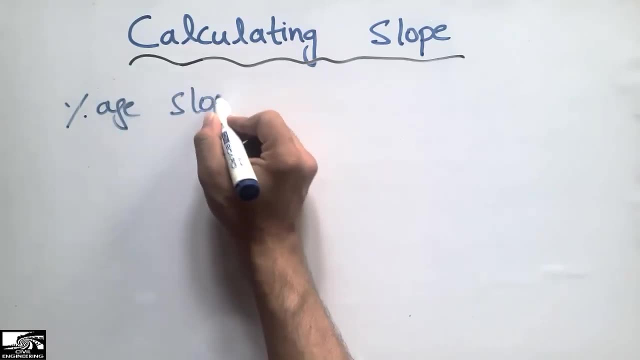 So there are two methods for determining the slope. One is the slope and the percentage slope. We find the slope and the percentage- the percentage slope, And the other one is the degree slope. We find the slope in terms of the degree slope. 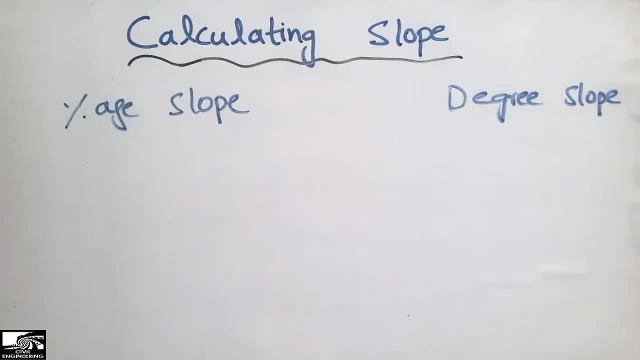 So let's consider this as a line, an intersection line, an inclined line, and we want to find the slope of this line. So consider the percentage slope of that particular line. the projection: there is a horizontal projection and this is the vertical projection of this line. 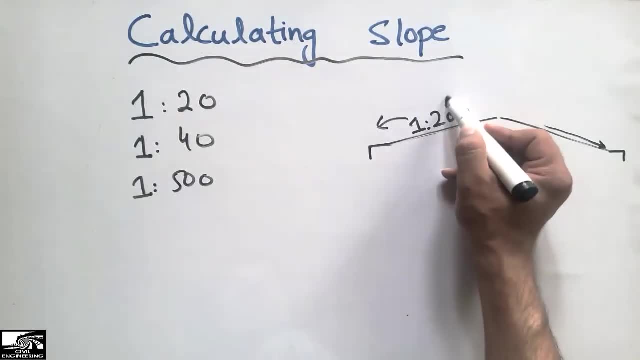 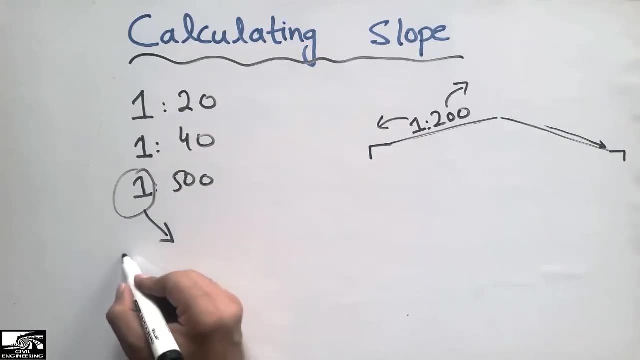 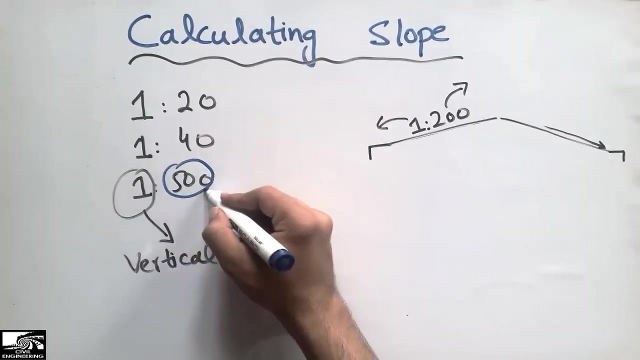 So what is the one value represent and what this 200 represent? The left side value. the left side value always represent the vertical portion of the line, the vertical portion right, While the right side value always shows the Horizontal portion of the line horizontal. 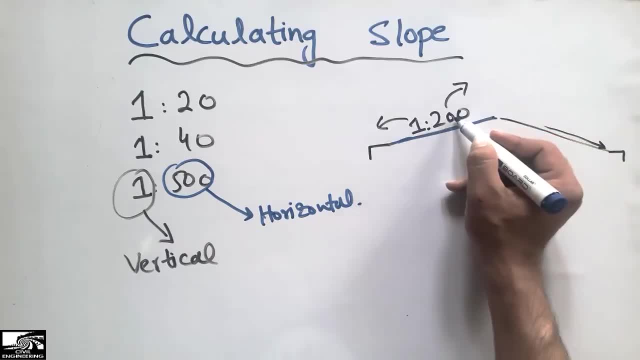 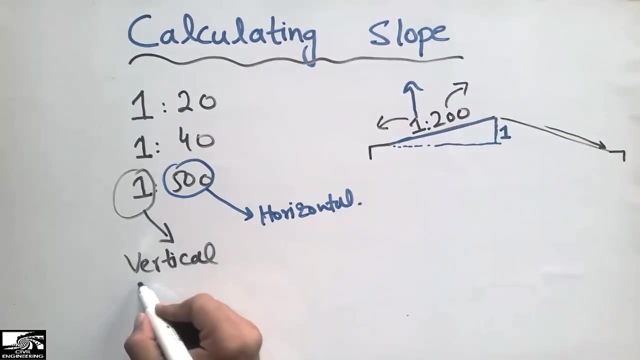 It means if this is the line having slope of 1, ratio, 200, it means that consider: this is the horizontal line and this is the vertical line of this line, vertical portion. So its vertical portion is 1, its vertical portion is 1, the left side 1 here, so I write 1, while the horizontal portion is 200, the right side is horizontal. 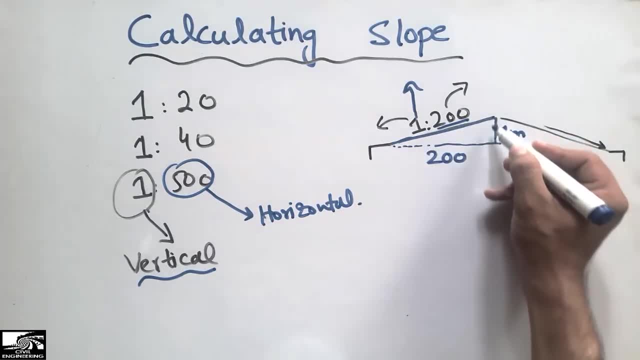 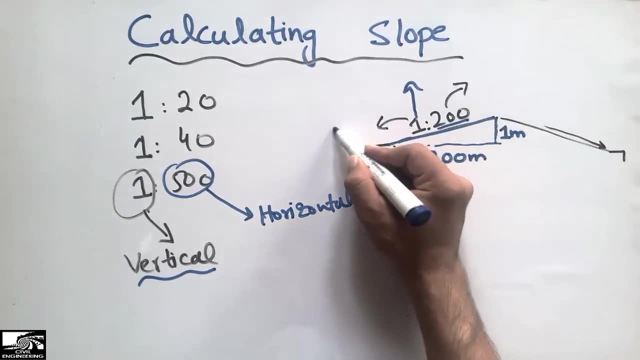 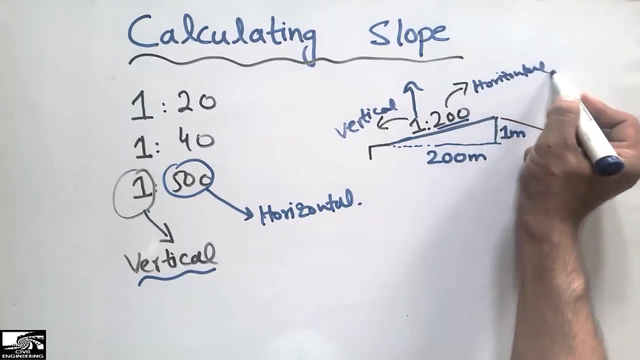 So it's 200,. it means if this is 1 meter high the line, so its horizontal distance will be 200 meter or length. This shows the vertical, while the right side value shows the horizontal. So this was all about the how we read the drawings. 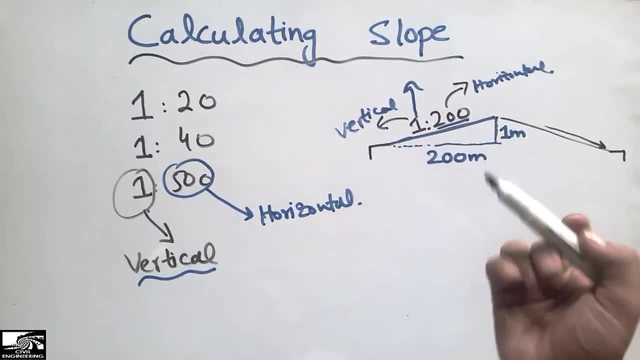 If the slope of any line or the intersection is given, so we can read these lines by knowing that this left side shows the horizontal length of the line And the right side value shows the vertical portion of the line. Similarly is the case with this value. 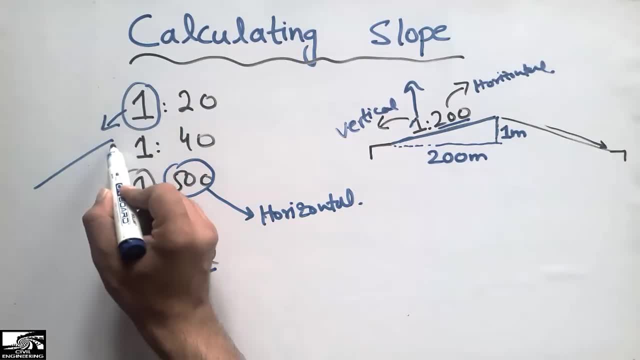 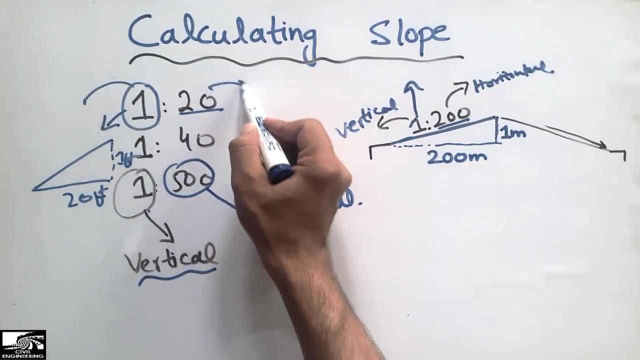 The one is the vertical line, if I consider this is the line. so one is the vertical line one here, while the 20 represent the horizontal length. It may be 20 foot, it may be 1 foot. So the one is a vertical foot, 1 foot and the horizontal is 20 foot. 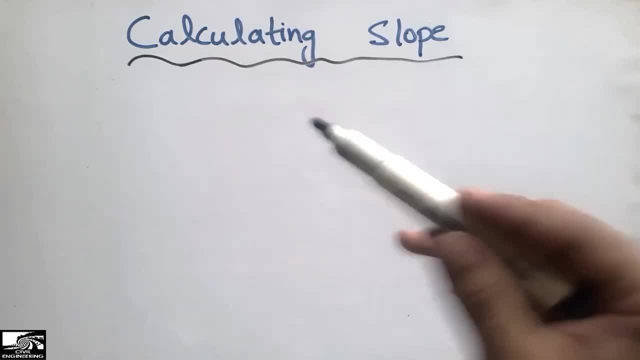 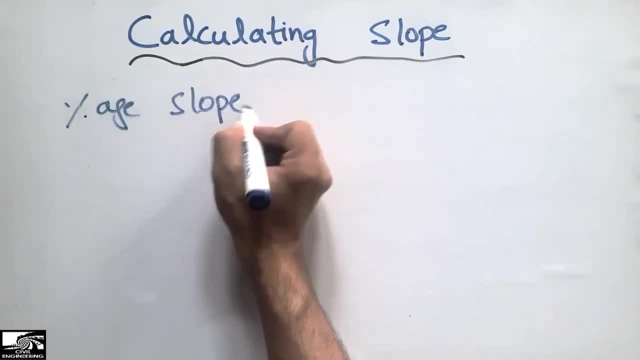 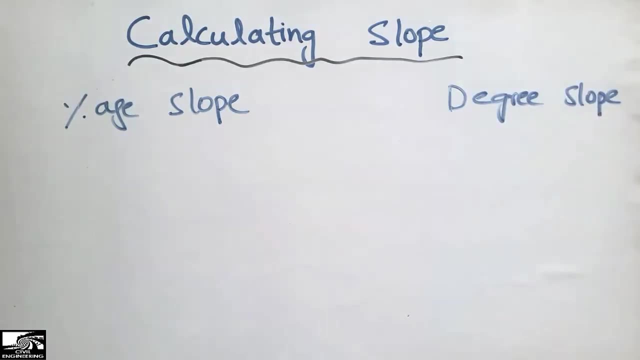 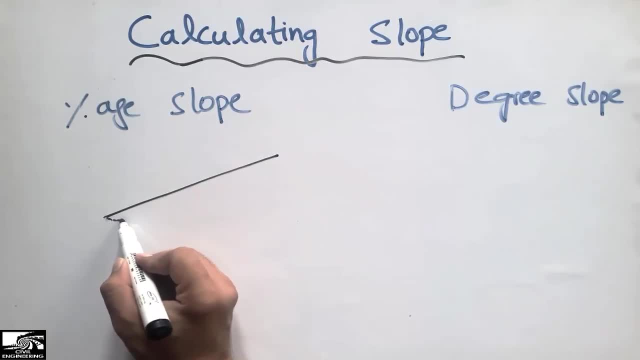 So consider the projection. this is a horizontal projection and this is the vertical projection of this line inclined line. So we call it rise. this is the rise portion and this is the run portion of this line. So the slope can be found out by dividing the rise by the run. 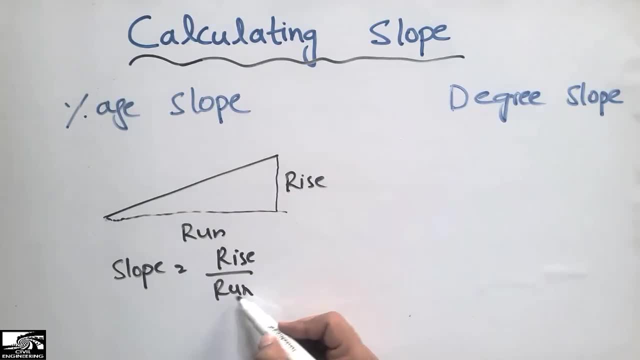 It means dividing the vertical portion by the horizontal portion, we get the slope of this line. If I consider this is 5 meter and I consider this is 2 meter. So dividing the 5 by 10, the rise by run, so we get the 0.5.. So it means the line, the slope of this line is now 0.5.. 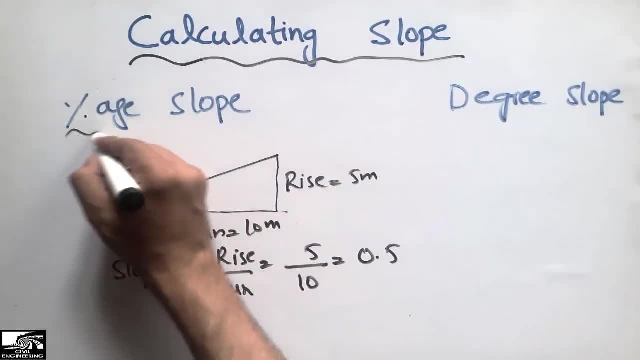 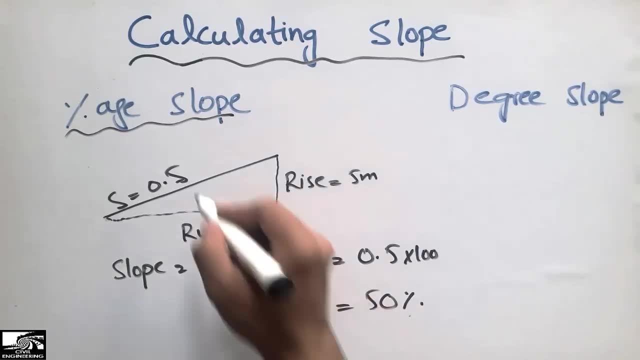 And we also call in terms of the percentage. this is the percentage slope. so we multiply it with the 100. What we get? We get 50%. It means the slope of this line is now 50% out of 100. So it's 50% rise in terms of the percentage. 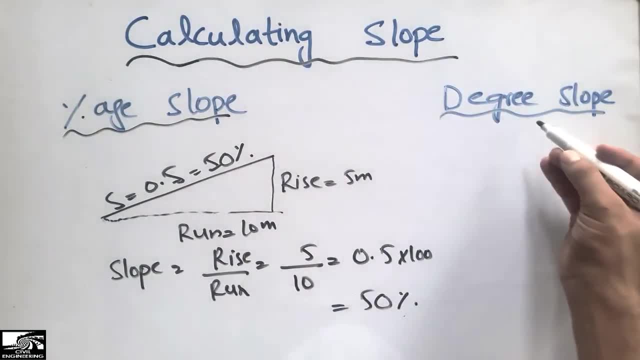 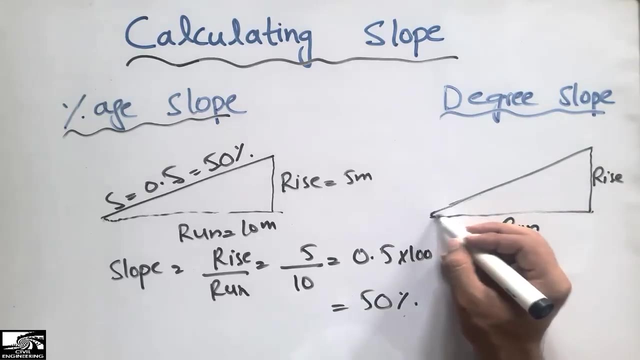 So this is the slope of this line. Now I want to show you that how we find the degree slope. So consider the same line, the inclined line, and this is the horizontal portion and this is the vertical portion. Or we can say, this is the rise portion and this is the run portion, and we want to find the slope in terms of the degree. This slope is unknown to us in terms of the degree. 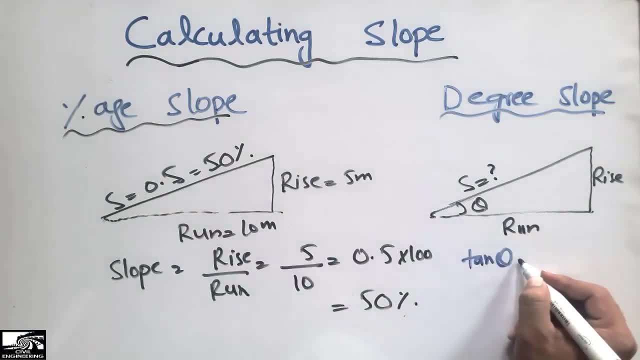 So, as we know that the tangent theta here tangent theta is equal to the slope, This slope is equal to the rise by run And now, dividing the rise by run, we get this slope in terms of the degree. For example, this is again 5 meter and this is 10 meter. 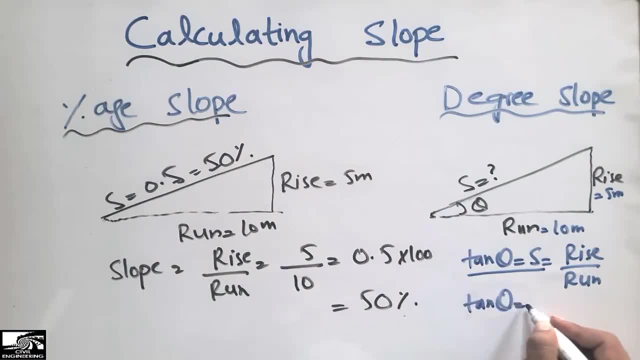 So the tangent theta is equal to the rise is 5 and run is 10.. Dividing these two it comes out to be 0.5.. And the tangent theta is equal to the tangent inverse and to 0.5, we get 26.5 degree. So it means this is now 26.5 degree. 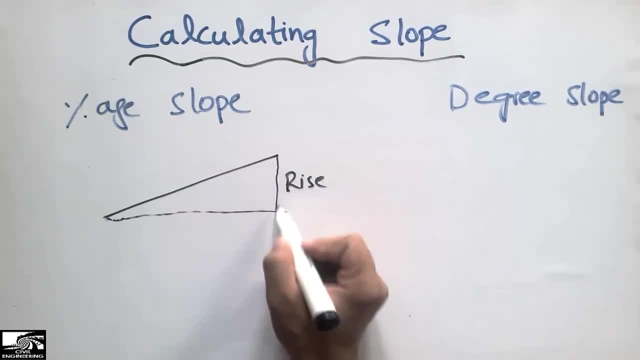 inclined line, so we call it rise. there is a rise portion and this is the run portion of this line. so the slope can be found out. by dividing the rise by the run means dividing the vertical portion by the horizontal portion, we get the slope of this line. 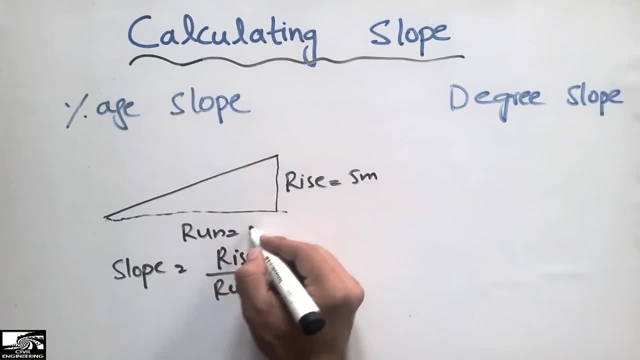 if I consider this is 5 meter and I consider this is 10 meter. so dividing the 5 by 10, the rise by run, so we get the point 5. so it means the line, the slope of this line, is now point 5. are we also call in terms of the percentage? this is: 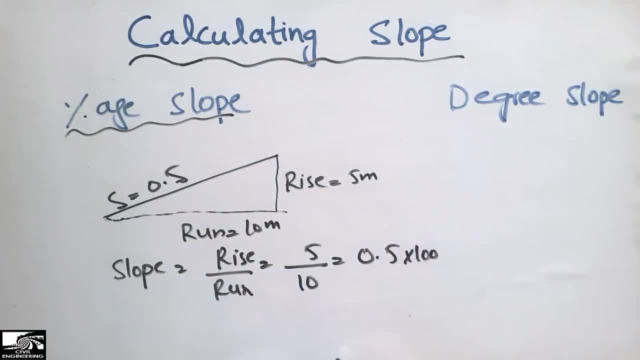 the percentage slope. so we multiply it with the hundred, what we get, we get 50%. it means the slope of this line is now 50% out of hundred. so it's 50% rise in terms of the percentage. So this is the slope of this line. Now I want: 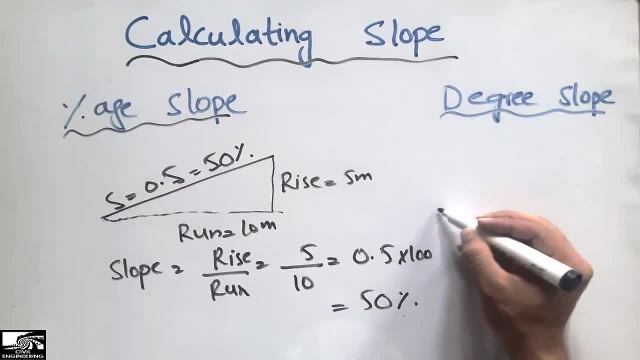 to show you that, how we find the degree slope. So consider the same line, the inclined line, and this is the horizontal portion and this is the vertical portion. or we can say this is the rise portion and this is the run portion, and we want to find the slope in terms of. 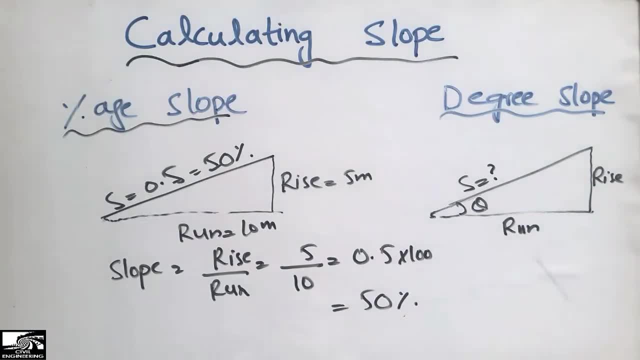 the degree. This slope is unknown to us in terms of the degree. So, as we know that the tangent theta- here the tangent theta is equal to the slope- is equal to the rise by run, And now, dividing the rise by run, we get the slope in terms of the degree. For example, 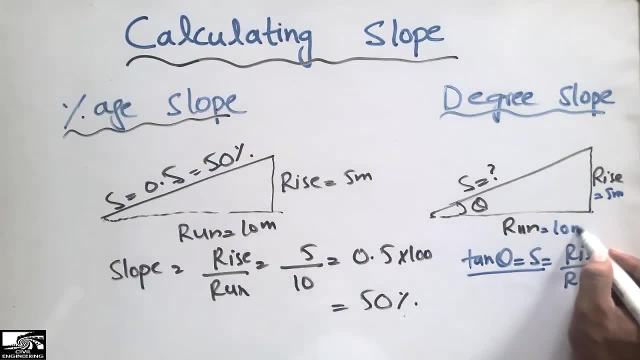 this is again 5 meter and this is 10 meter. So the tangent theta is equal to the rise is 5 and run is 10.. Dividing these two it comes out to be 0.5.. And the tangent theta is equal to the tangent inverse and to 0.5 we get 26.5 degree. So 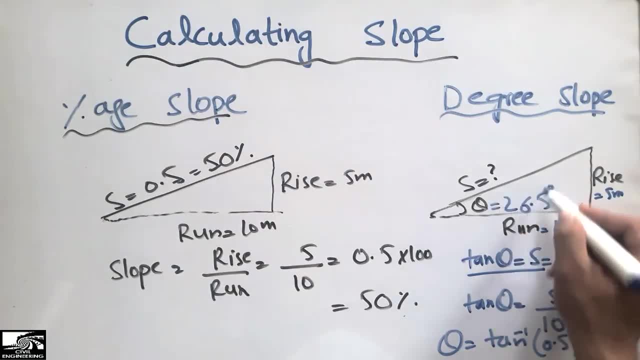 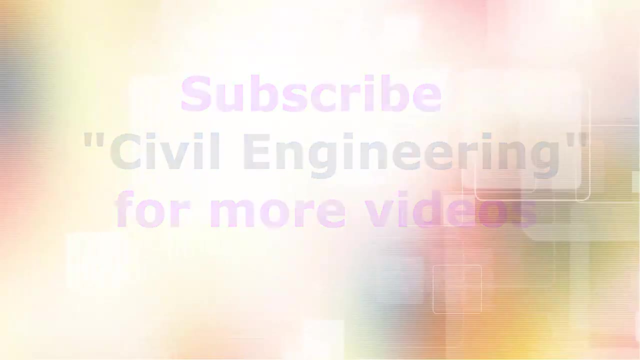 it means this is now 26.5 degree. So the slope is now. we can say the slope of this line is now 26.5 degree.